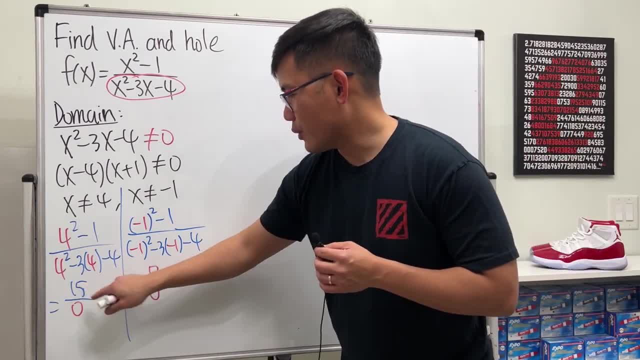 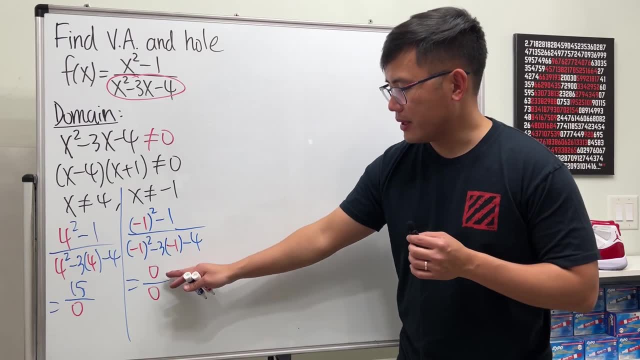 work that out, we also get 0.. All right, so we have two very different behaviors. The first one is a non-zero number over 0. The second one is 0 over 0. So what's the conclusion? This one right. 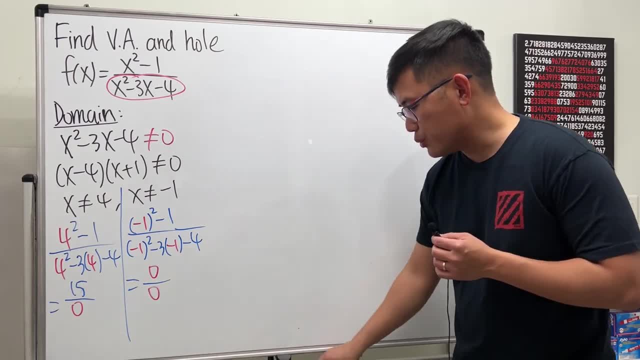 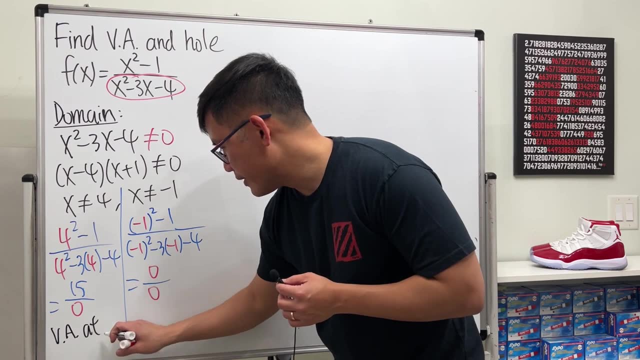 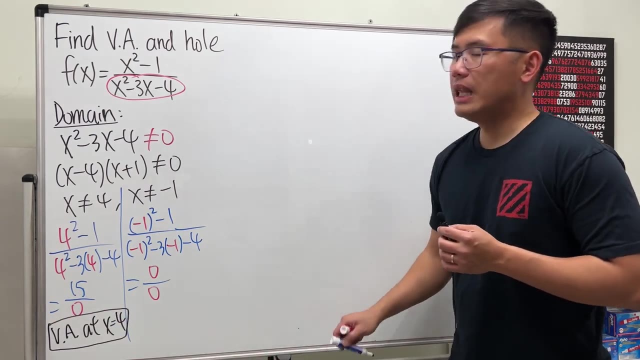 here in fact we cannot conclude anything yet but this one- we can actually conclude that we have a vertical isotope. So right here we have a vertical isotope, and we have a vertical isotope. Right here I can say: we have a vertical isotope at x equals 4.. All right, and then now let me 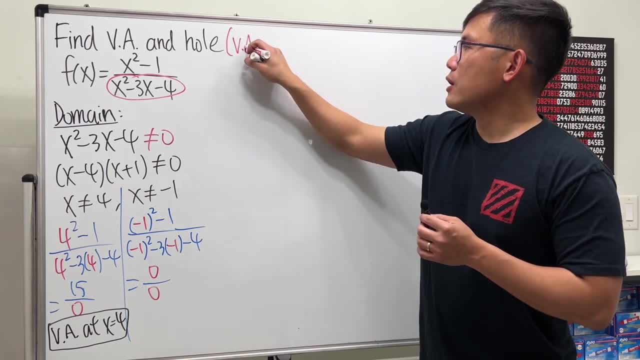 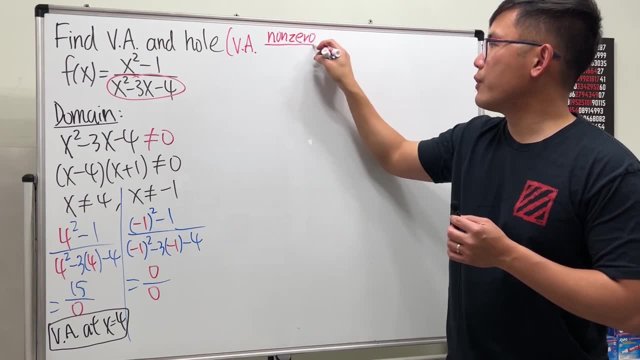 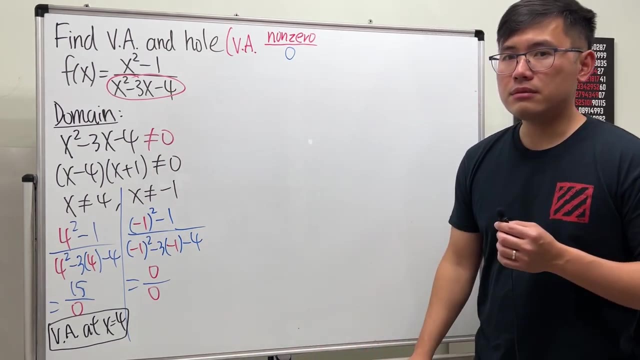 write down some notes for you guys. For the vertical isotope, this is the situation that we have a non-zero number on the top over a 0 on the bottom, guaranteed Whenever you have that vertical isotope. when we have that Done. 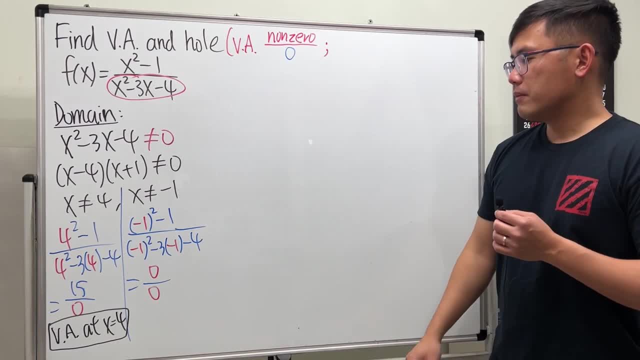 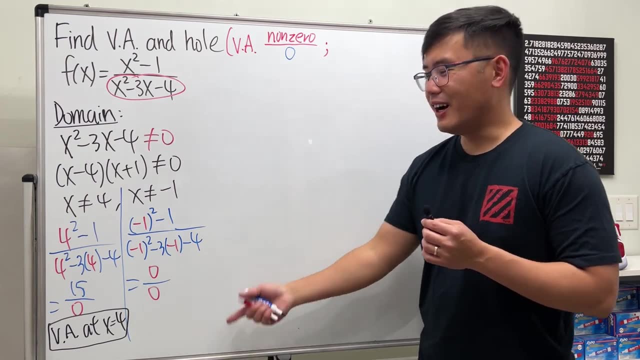 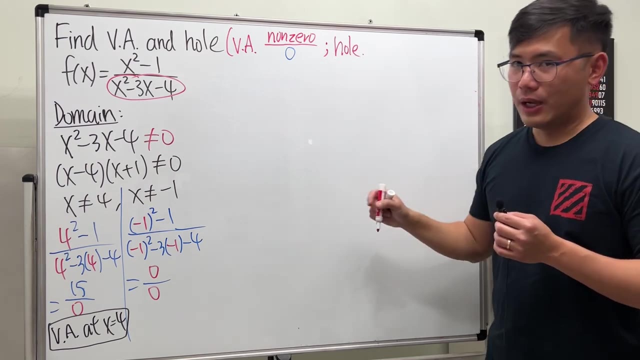 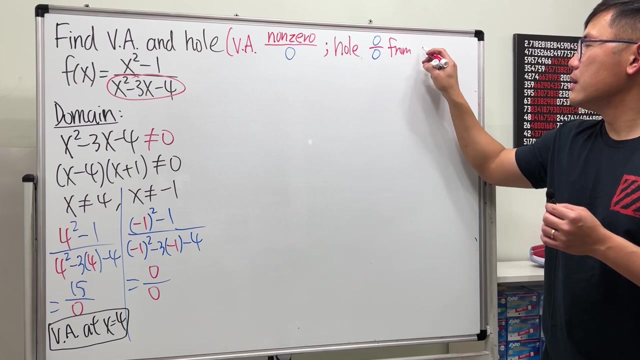 Right Now, what's 0 for 0, though This right here is technically just a candidate of being a whole of the graph, So let me write this down right here for you guys, In order for us to get a role. how do we do it? Firstly, we get 0 over zero from the original. 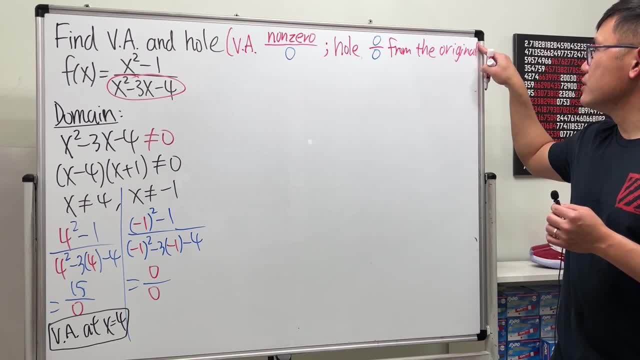 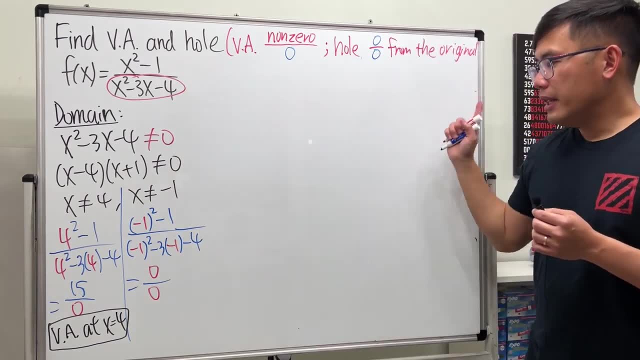 meaning that you don't- あたたた ~~~, reduce anything, just from the original, which we did right here. right, because that's what we did. well, in fact, this is not enough. you also have to plug in negative 1 into the reduced version. 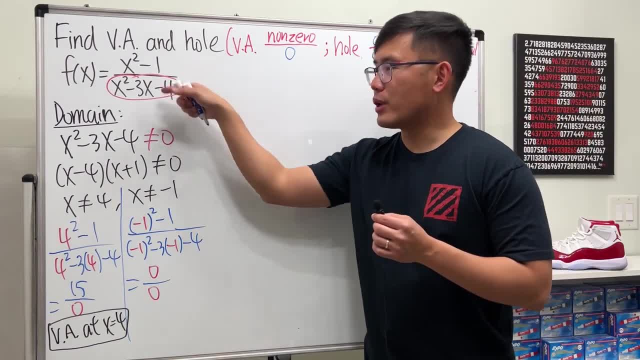 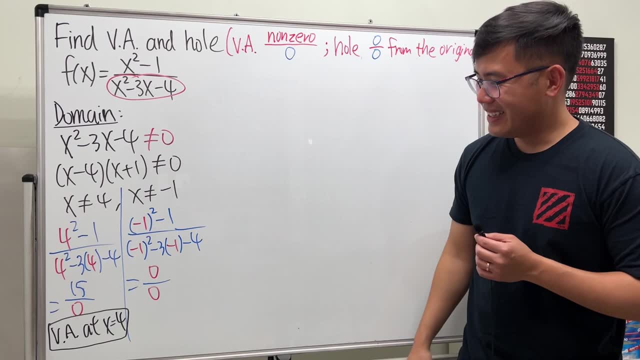 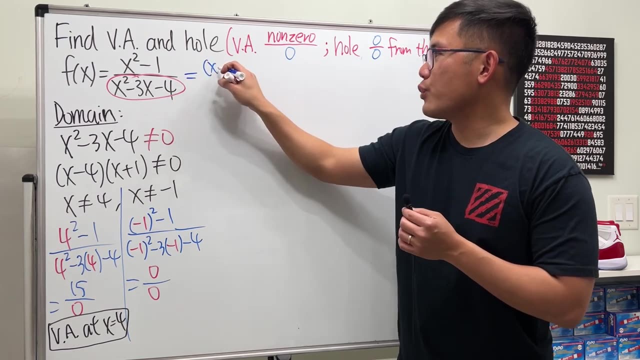 whenever you get 0 over 0. in fact, this right here can be reduced, trust me, because of the factory. zero technically, but you can also trust me. all right, let's go back here, and the factory can source himself. look on the top. we can factor it as the difference of two squares. we get x minus 1. 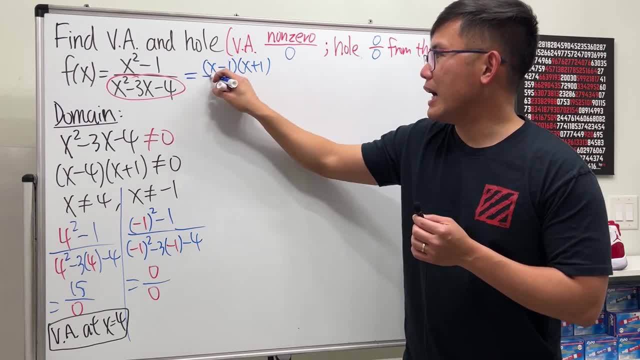 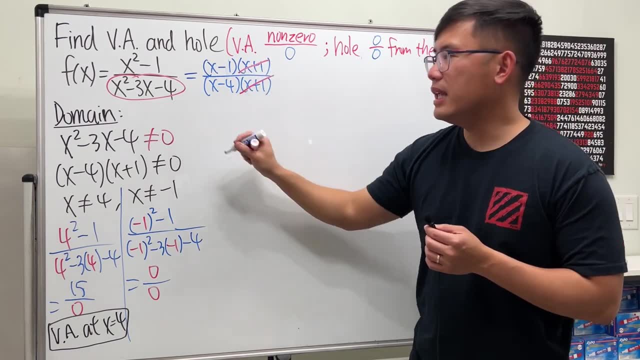 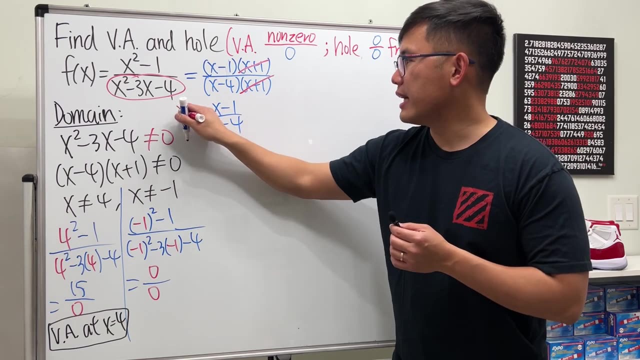 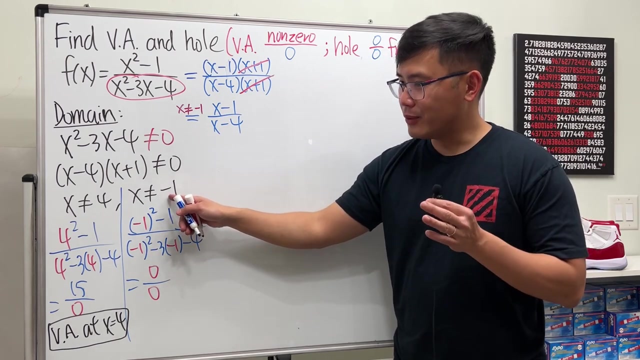 times x plus 1, and then on the bottom we have x minus 4 times x plus 1. this and that can cancel, and we know this is equal to x minus 1 over x minus 4, under the condition that x is not equal to negative 1.. okay, what we do have now, what we have to do. 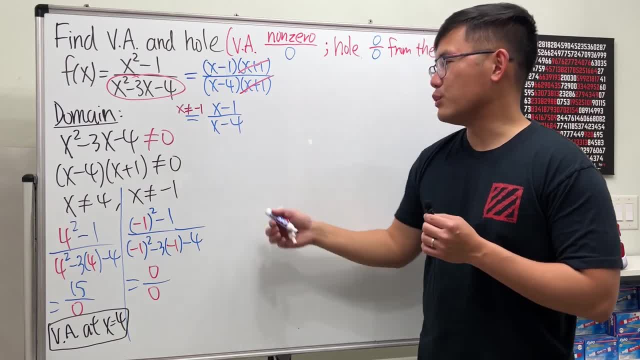 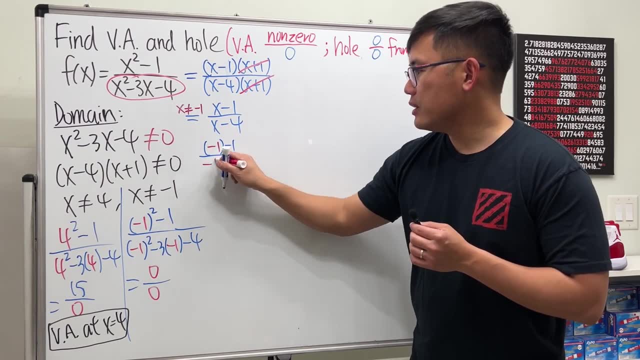 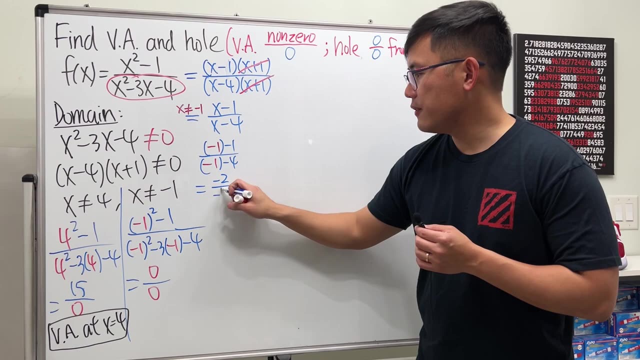 now is to put negative 1 into the reduced version and see what happens. let's see, we will get negative 1 minus 1 over negative 1 minus 4, and this, right here, gives us negative 2 on the top over negative 5 on the bottom, which is just a nice number. so, in fact, here is the detail. 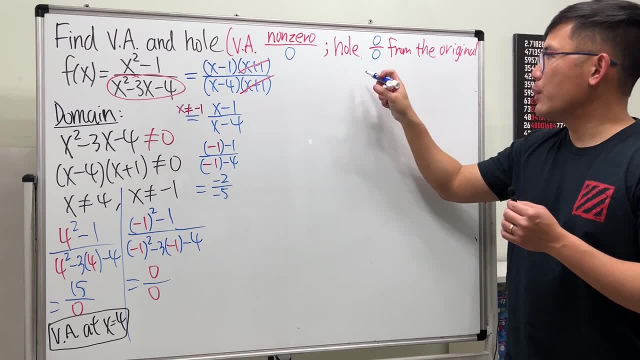 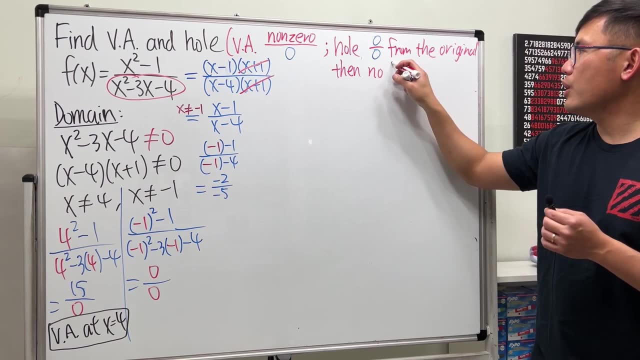 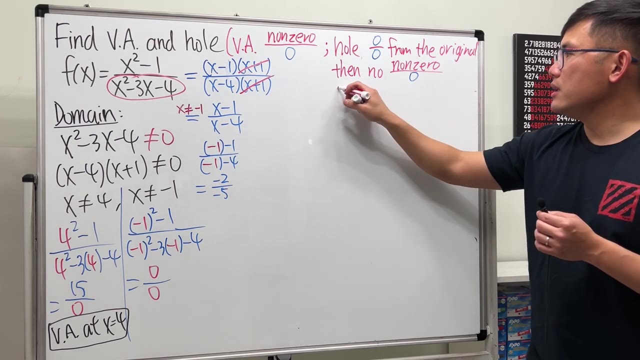 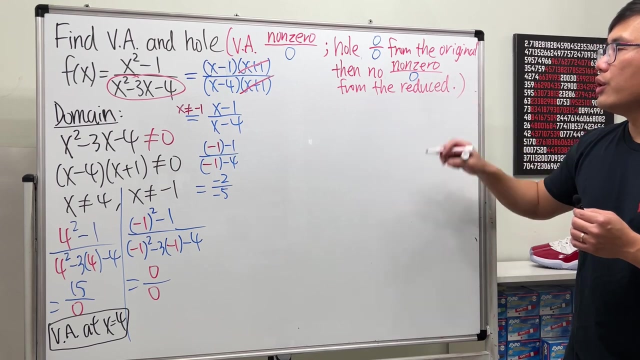 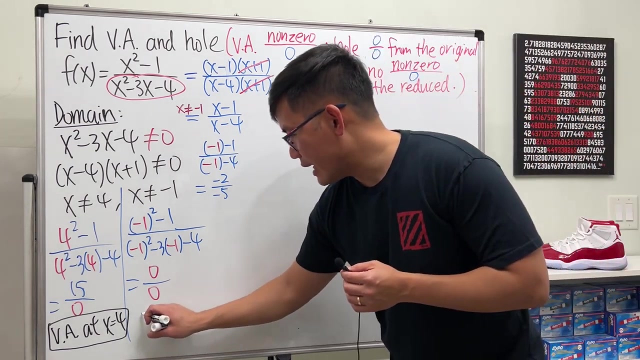 if you get 0 over 0 from the original and then i will have to say: then no, zero, no, non-zero over 0 from the reduced expression, then you will have a hole on the open on the graph. so right here we can draw a conclusion that we have a hole at x equals. 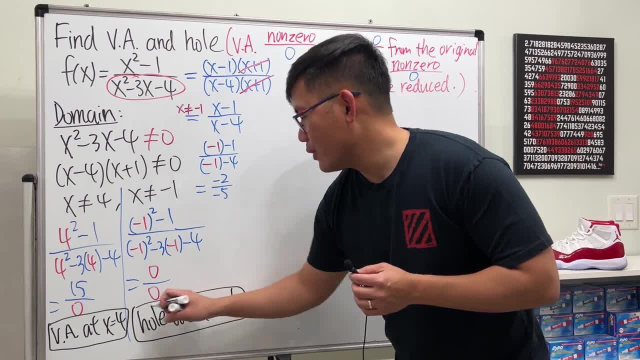 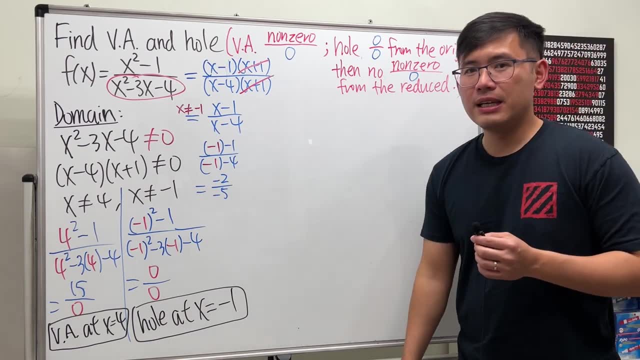 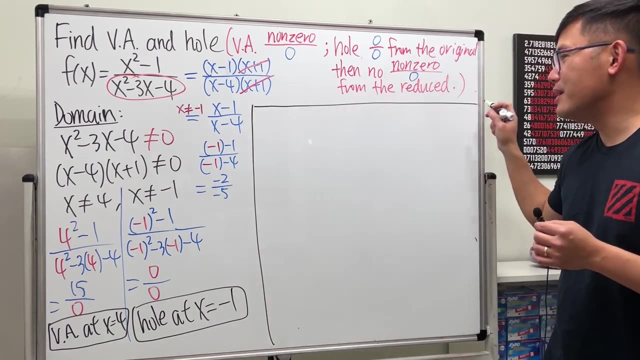 negative: 1.. yay, we are done. but maybe some of you guys notice already why the elite space like this right here. right, because i want to show you guys this right here real quick, because this kind of things can be extremely tricky. all right, let me demonstrate this idea real quick, all right so 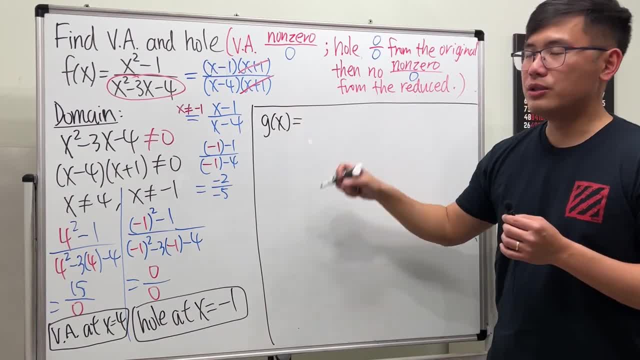 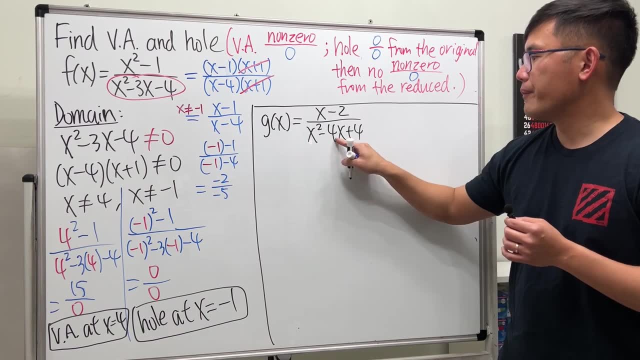 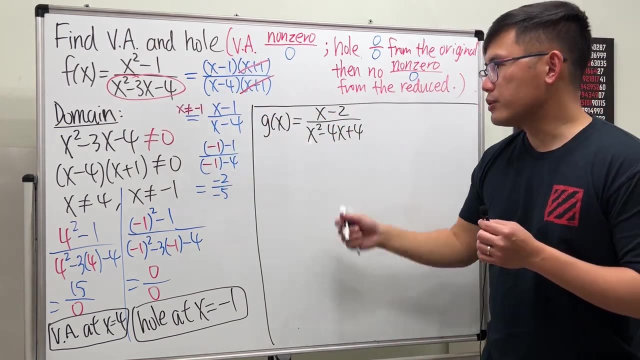 let's consider another function. let's say g of x, and for this one let me just tell you if we have x-2 over x, squared minus 4x plus 4.. let's go ahead and identify the vertical isotope and the whole of the graph of this function, and to do so again, we are just 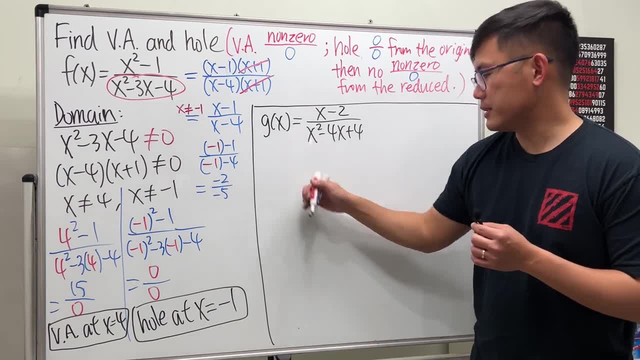 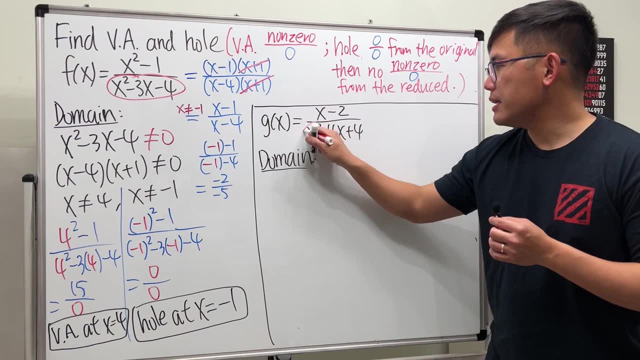 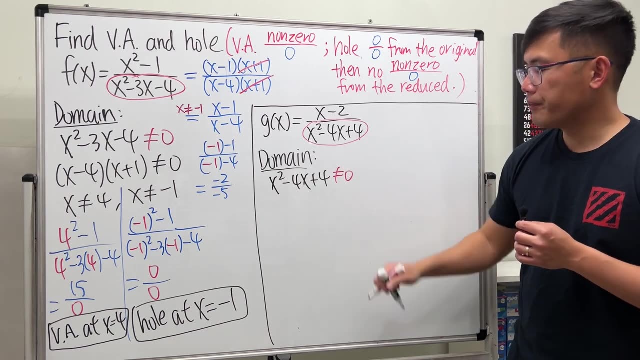 going to look for the candidates first and that's to find the domain first. so let's pay attention to the denominator not being equal to zero. so x-square minus 4x plus 4, or put in, not equal to 0. Factor it, we get x minus 2 times x minus 2,. 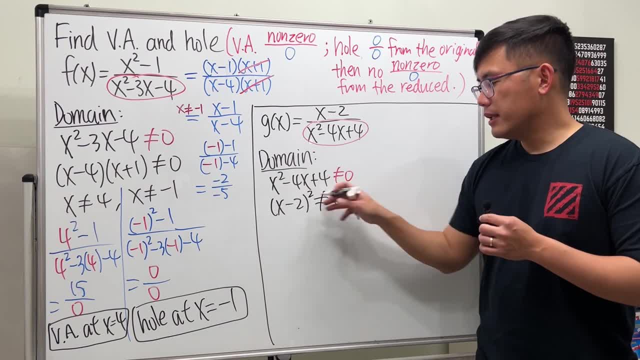 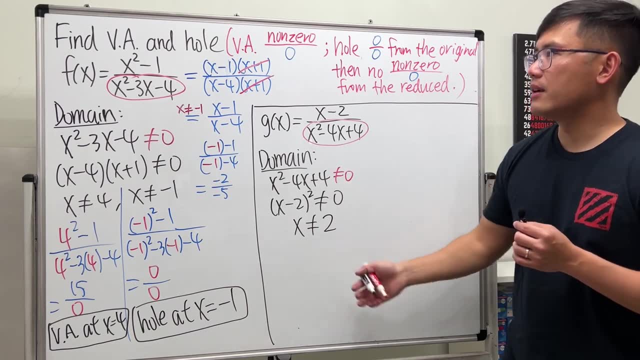 which is x minus 2 squared not equal to 0.. This means x cannot be equal to 2.. And this right here will tell us the candidate for the vertical acetone or the hole, But which one is which? Let's go ahead and do what we did. 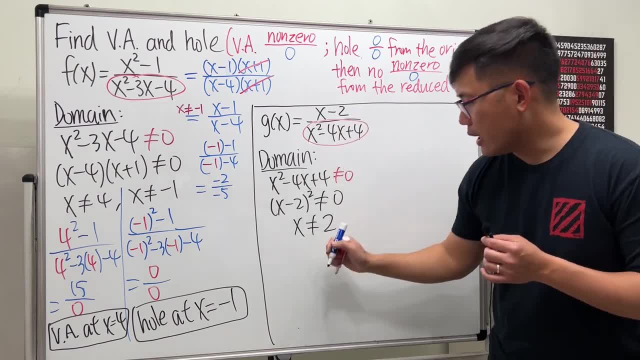 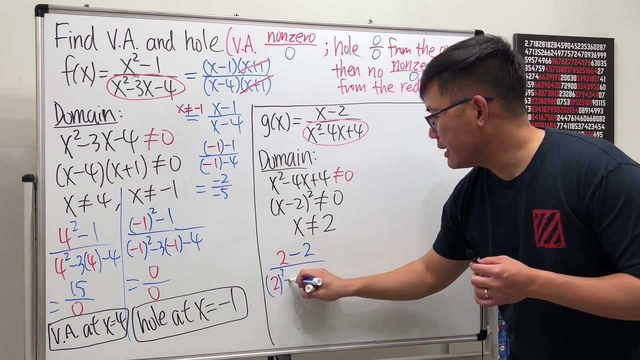 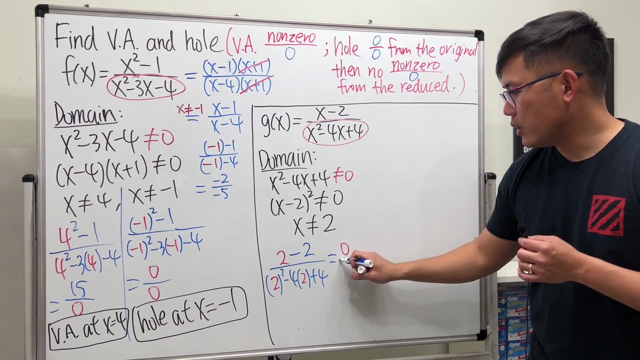 First plug in 2 into the original. So we are going to get 2 minus 2 over 2, squared minus 4 times 2, and then plus 4.. For this one on the top, we get 0, on the bottom we also get 0.. 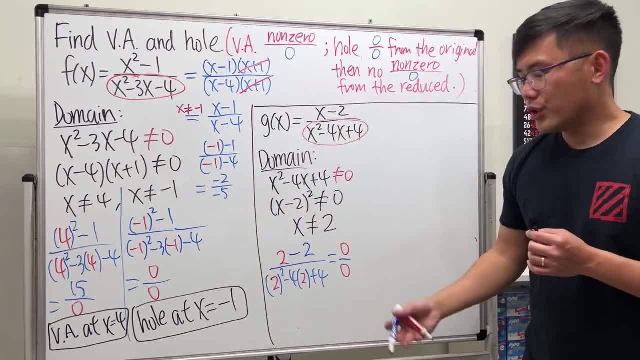 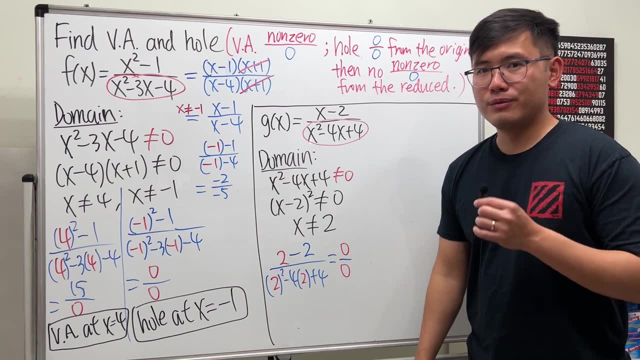 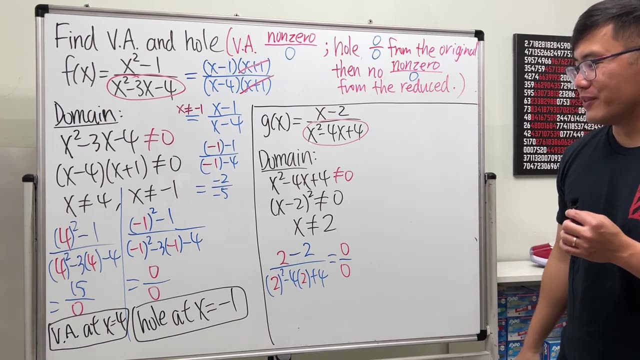 So what do we get? Is this a hole on the graph at x equals 2? No, Why? Because of this? Why Because it's tricky. So be really careful with that When you get 0 over 0, when you plug into the original. 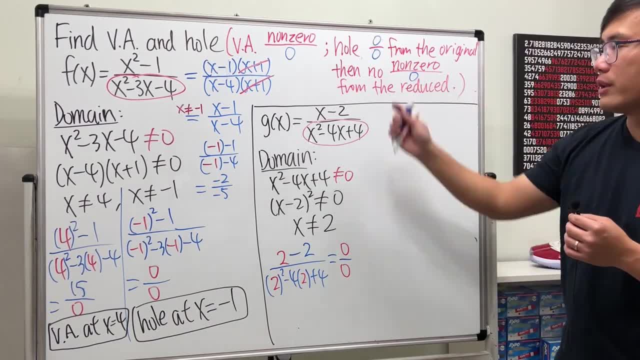 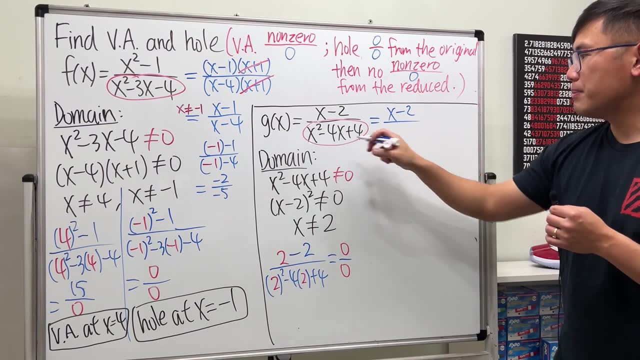 it's just a candidate being a hole on the graph. Now look at this. We can factor it. On the top, it's just x minus 2.. On the bottom we get x minus 2 squared, which is x minus 2 times x minus 2.. 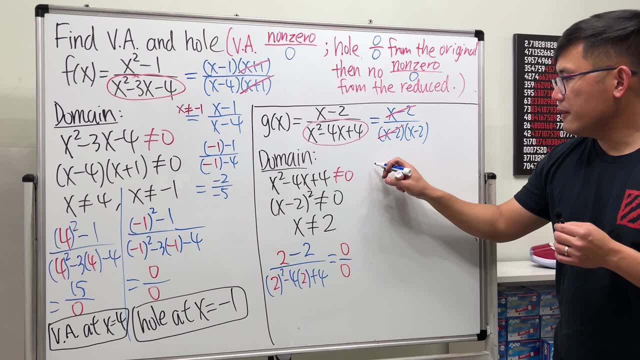 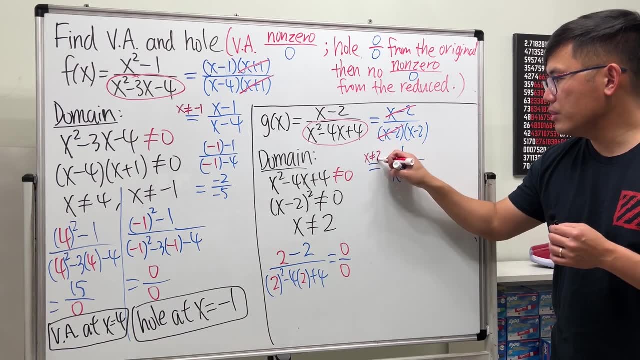 Well, you see that we can cancel one of these And in fact we get 1 on the top over x minus 2. And again, that's denote that x cannot be equal to 2.. Now, if we put 2 into the reduced version, 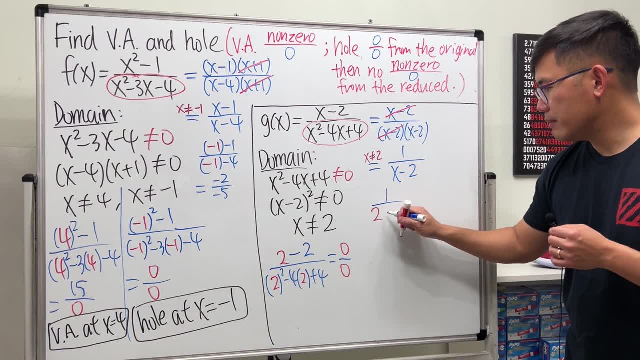 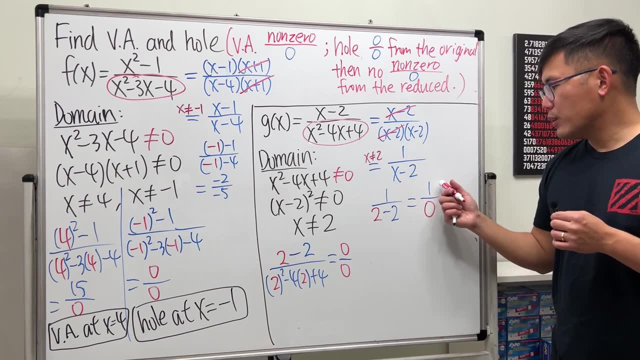 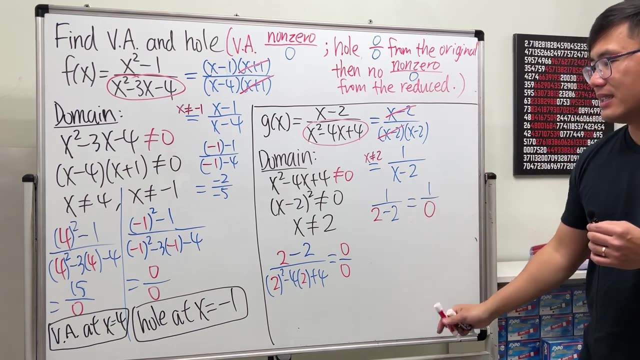 what do we get? We get 1 over 2 minus 2, which is 1 over 0.. If you still end up with a non-zero number over 0 from the reduced expression, in fact, you will end up with a vertical acetone. 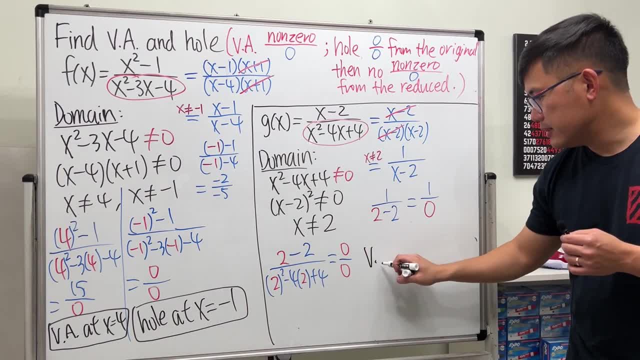 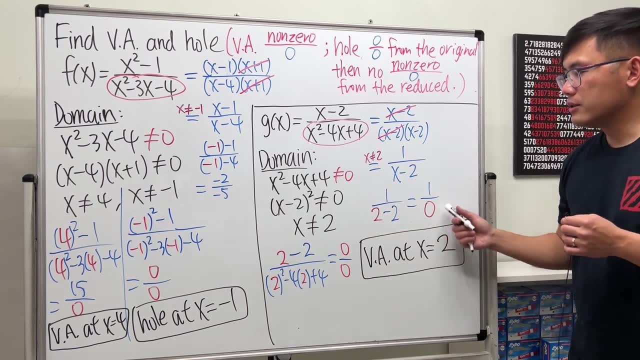 You end up with a vertical acetone still. So for this situation, we will have a vertical acetone at x equals 2. So be really careful. I know it's tricky, I know it's hard. Together we can do it. 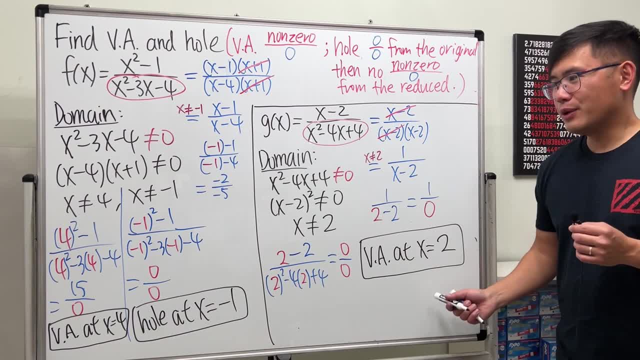 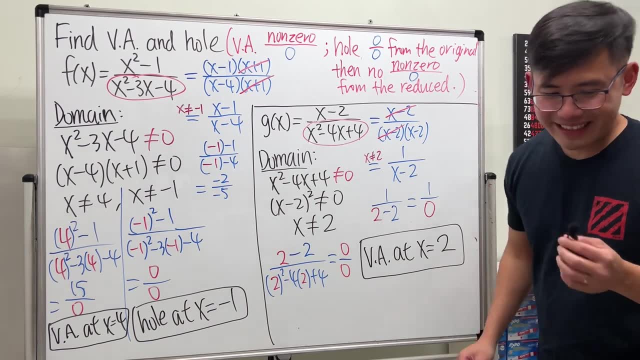 just with some practice with it. Let me know if you guys have any questions. I'll be happy to make more videos for you guys with similar questions, But hopefully this right here is clear. That's it.